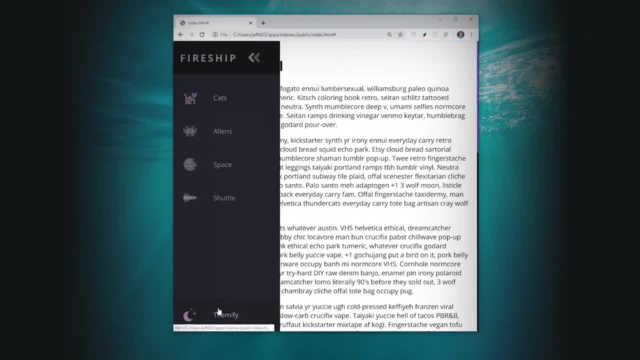 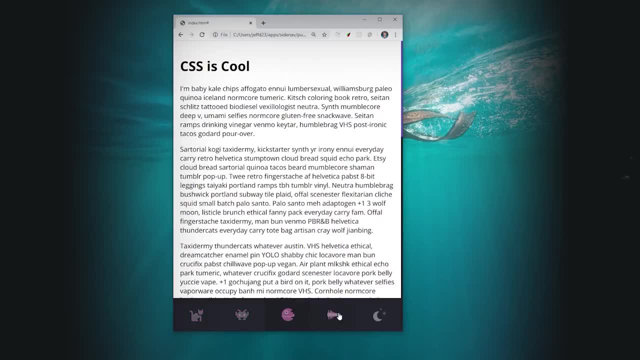 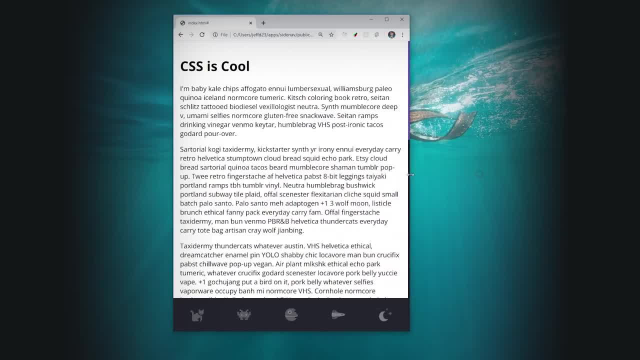 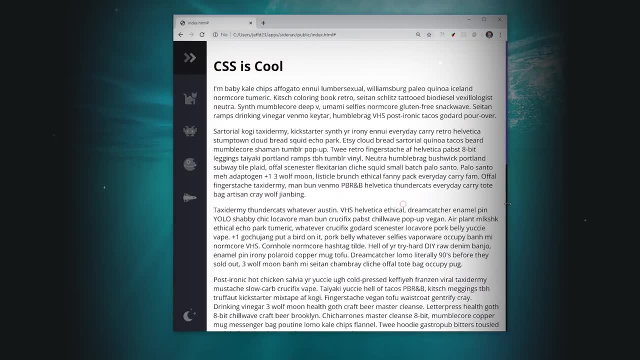 down and we'll also be using Flexbox to lay everything out, which makes it really easy to convert a column into a row. So we'll use a media query for small devices to take the nav bar and fix it to the bottom, And that should provide a much better experience on mobile. 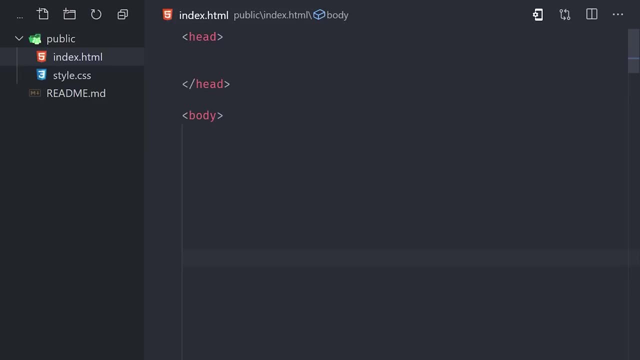 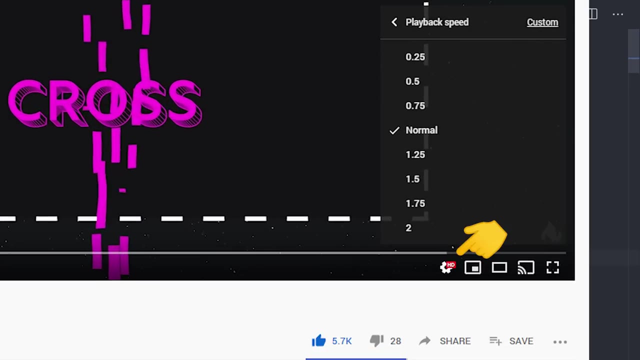 assuming that your app is intended to be used in portrait mode. That gives us a good starting point, so let's go ahead and jump right into the code Now. this video is designed for you to follow along, but we'll be moving at a very quick pace, so feel free to slow down the playback speed or 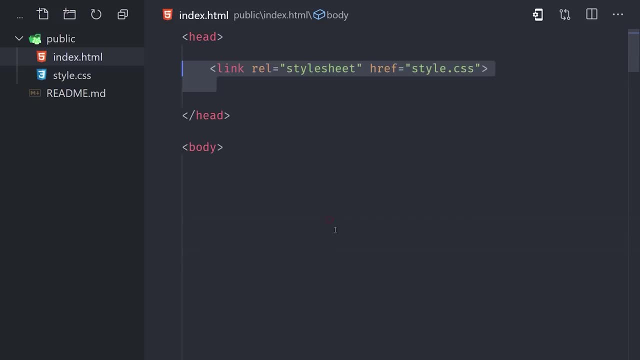 pause if necessary. You'll notice I have an index HTML file and a stylecss file which is rough for reference, in the head of that HTML document And you'll also notice I have a custom font from Google Fonts. Feel free to use whatever font you prefer. Now, moving on to the body of the HTML, 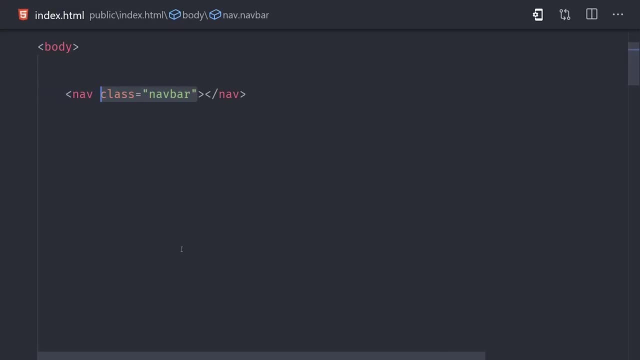 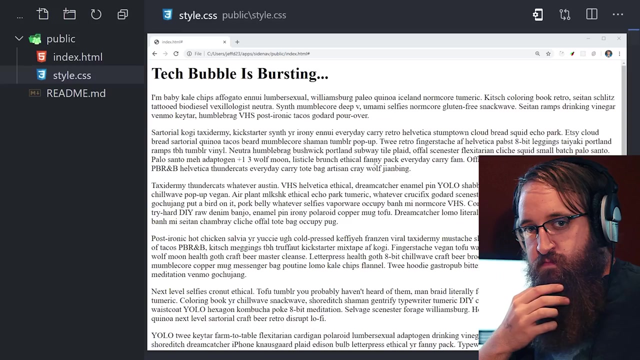 we have a nav element, which is the main thing we're building today. Then, alongside that, we have a main element to hold the main content of the page, and right now it's just filled up with a bunch of hipster ipsa. Currently, our HTML is completely unstyled. Let's start by setting a few. 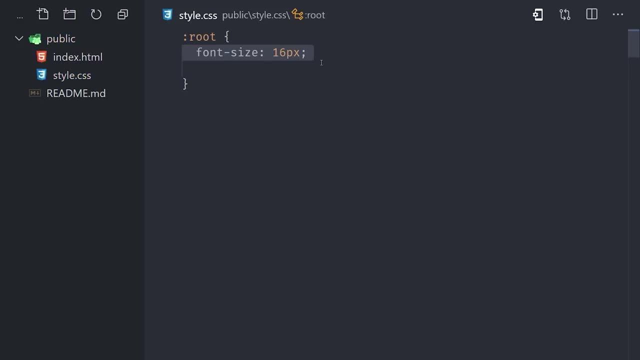 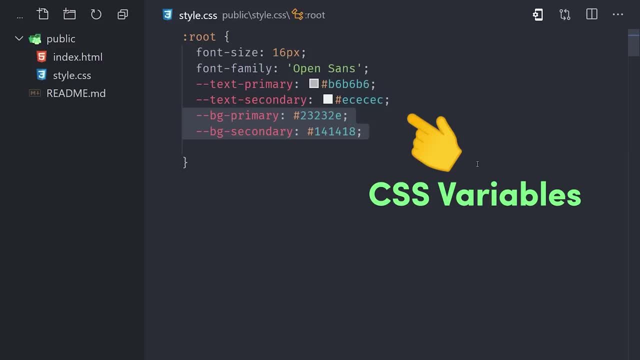 the theme of the application. They always start with a double hyphen and when you define them in the root, they can be used throughout all of your other CSS classes. This makes it really easy to swap different colors and themes on the fly, and you can always override values in lower classes. 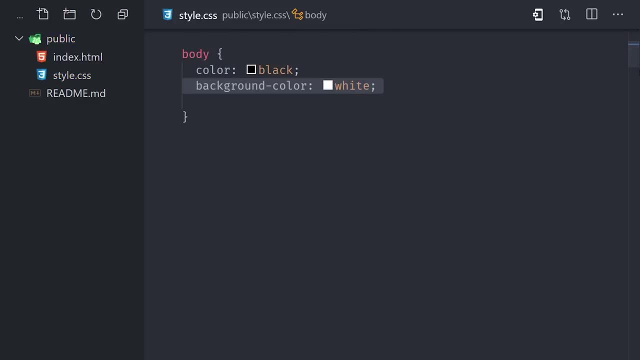 as needed. Next, we'll set a couple of fixed values in the body and eliminate any margin or padding In the main element. we'll set a margin on the left so that our navbar doesn't overlap the main content. We'll set that to 5rem. 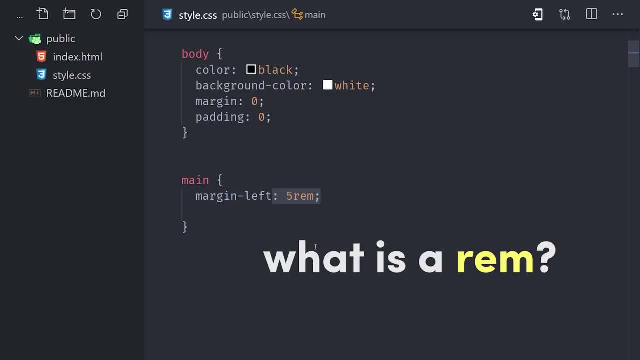 but you might be wondering what is a rem unit? It's a unit that is relative to the font size on the root element. A few seconds ago we set the font size on the root element to 16 pixels and that means 5rem in this case is equal to 16 times 5, or 80 pixels. Relative units like 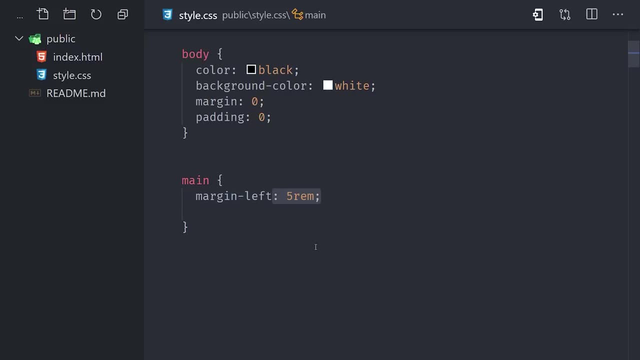 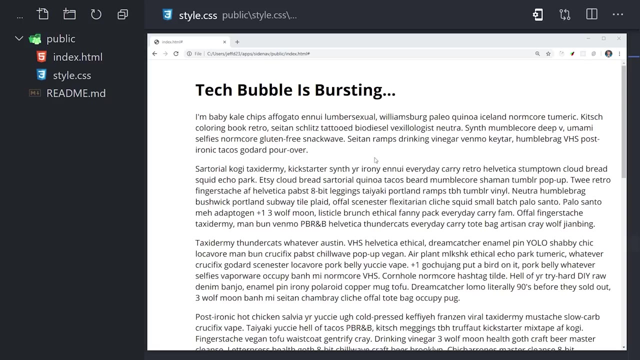 this can be very useful because if you go and change your font size, it means that everything will stay proportional to that font size, so you don't have to go and manually update pixel values. Now, if we go ahead and load our HTML in a browser, you can see we have some white space on the left. 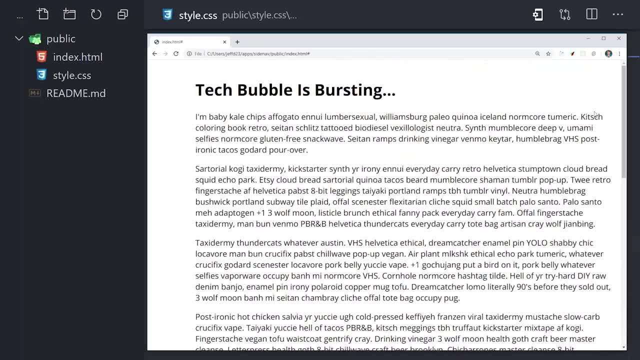 side where our navbar will be. We can also set the font size on the root element to 16px, and we'll set the font size on the left side where our navbar will sit. But first there's something that's bothering me, and that's this default scrollbar that comes with. 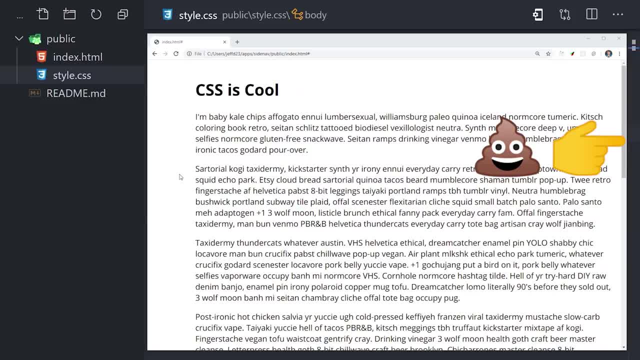 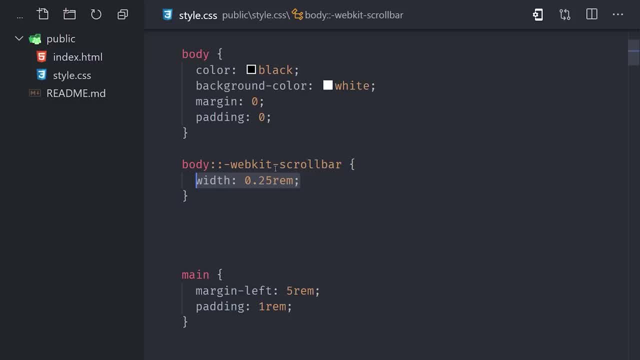 the browser. It's especially ugly with this type of layout. so how do we customize the browser's scrollbar? We can style it by targeting a pseudo-element on the element with the scrollbar. In our case that's the body element, and we can use WebKit's scrollbar to adjust the width. 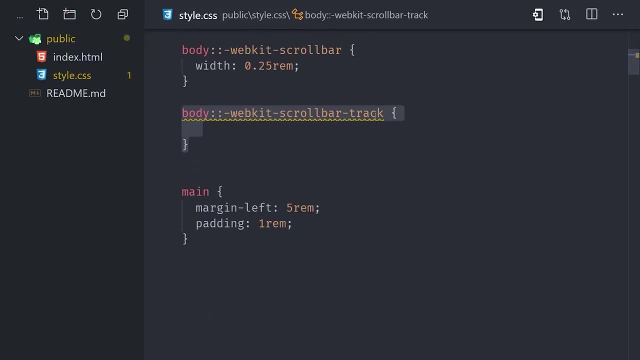 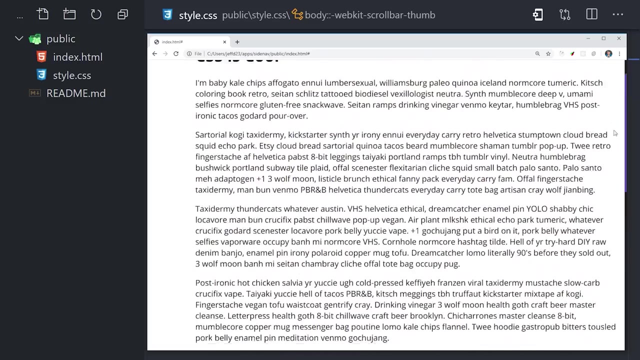 Then we can use a separate pseudo-element to change the background of the track and then yet another to change the color of the actual thumb that moves along that track, And just like that, we now have a much better looking scrollbar on the body. Now we're ready to start building the navbar. 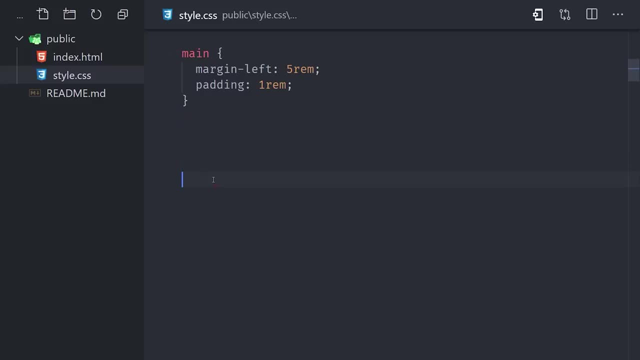 and the first thing we'll want to do is make it fill the available space here on the left. We'll start by setting the width property as 5rem and notice how that matches the margin left we set on the main element. Then we'll set the height as 100vh units. Vh is also a relative unit. 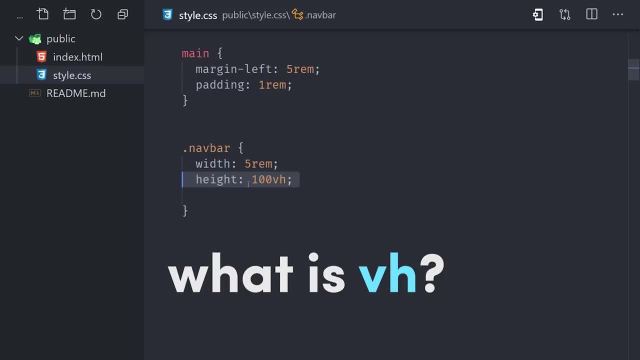 but it's relative to the size of the viewport. 100 will always fill up 100% of the height and will react accordingly. if the user changes the size of the browser window From there, we'll give it a position of fixed, so it stays in the same place no matter where the user scrolls to. 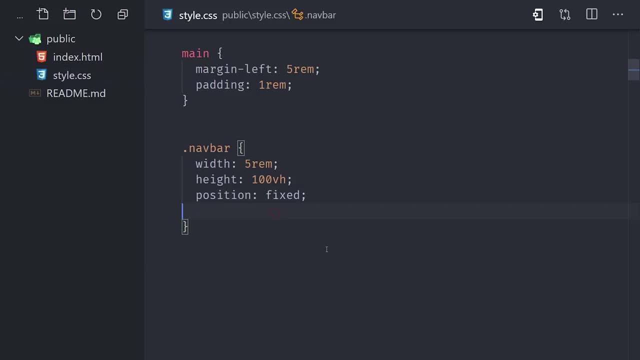 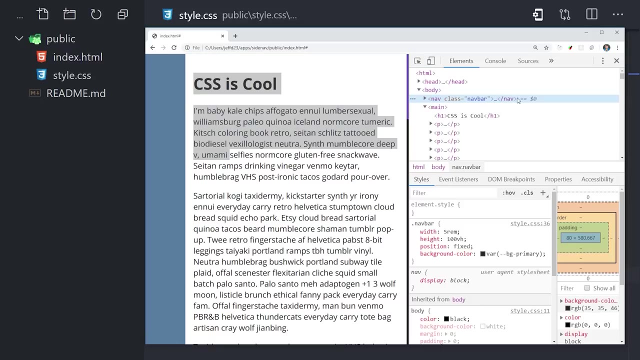 on the screen And then we'll tell it to use one of our CSS variables for the background color, using the var keyword. So now that our main navbar is in place, we need to fill it up with some more HTML. I'll do this following similar conventions to what you would find in something like Twitter. 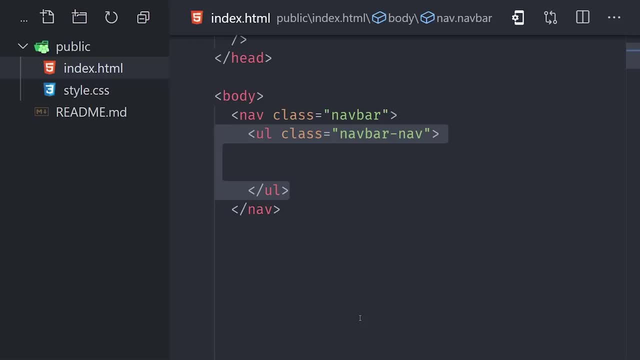 Bootstrap. We'll start with an unordered list and then add an individual list item for each individual item in the menu. Inside of each list item we'll have an element or a link, and inside that link we'll have some text, along with an. 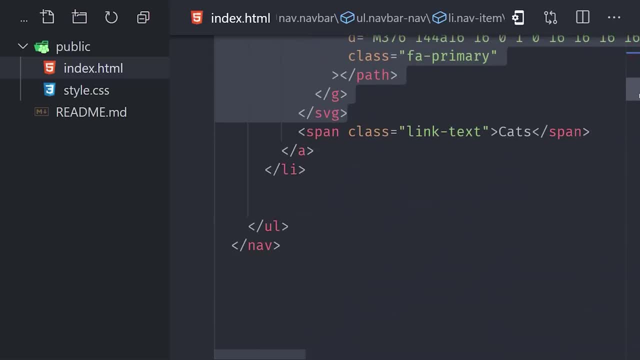 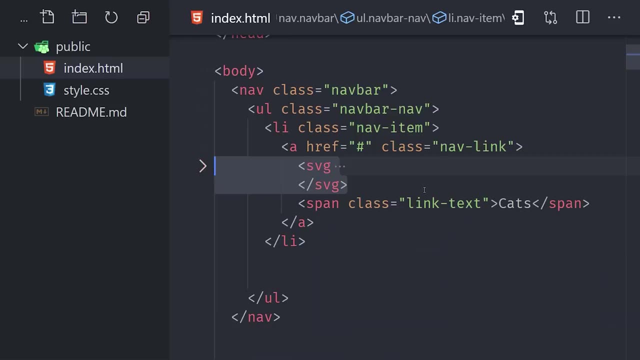 SVG icon. The actual icon itself comes from Font Awesome. You can find a bunch of free icons there and they just released a bunch of new duotone icons, or you can create your own from scratch. The special thing you'll notice about the duotone icons is that the paths inside the SVG graphic 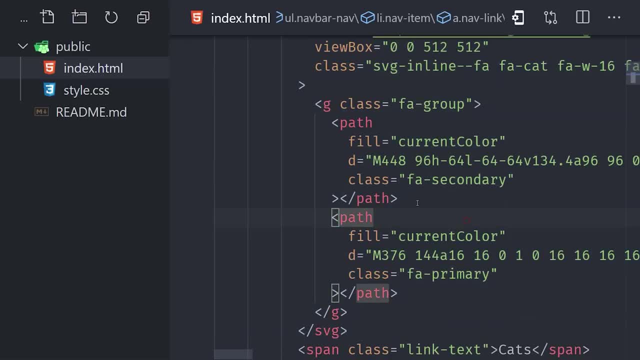 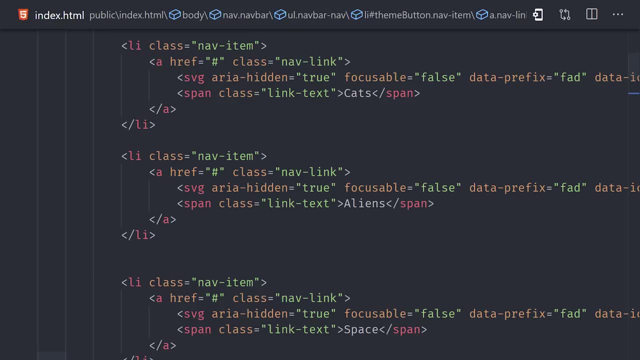 have a class of fa-secondary or fa-primary And we can target those classes to change the color of different parts of the SVG. Now I'm adding a few more list items to the menu. they follow the exact same format. the only difference is the SVG icon and the link text. 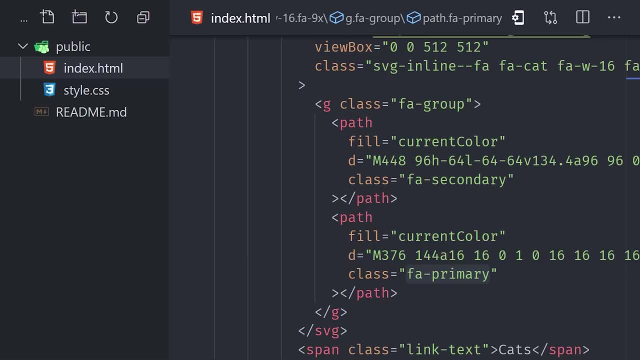 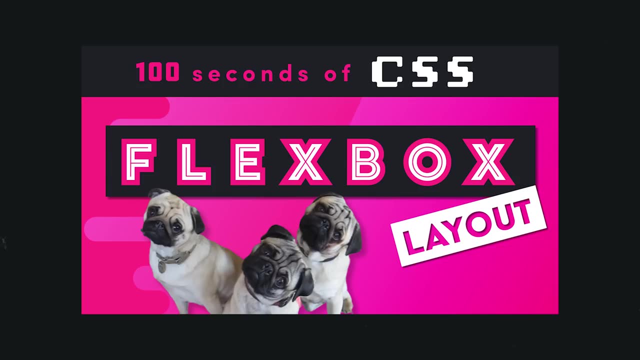 Feel free to copy and paste the markup from the GitHub repo. Now, at this point, our navbar doesn't look very good. What we need to do is use flexbox to position these items directly in the middle of the column. If you have no idea what flexbox is, you might. 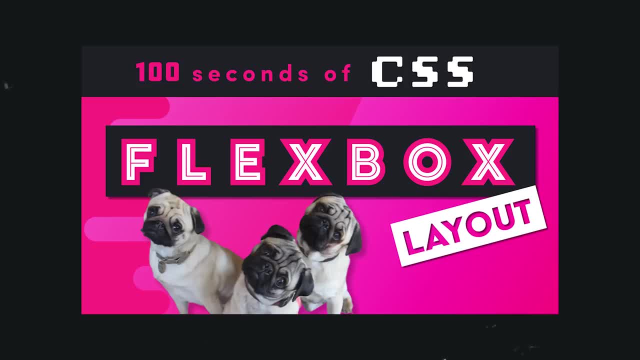 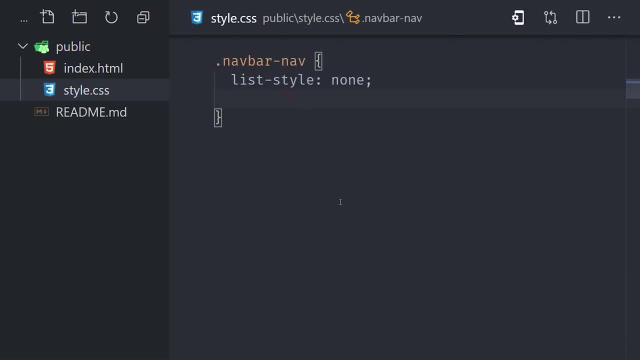 want to pause this video and check out my 100 seconds of code video on that topic to get an introduction. Our main goal is to create a column with flexbox so the items flow from top to bottom. The unordered list in the HTML will be our flex container. We'll remove the default list style. 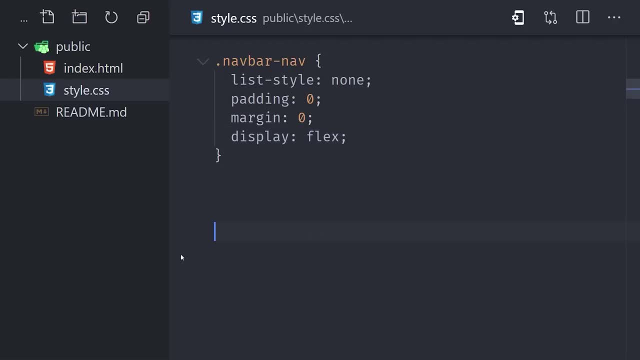 the padding and the margin and then set the display property to flex. By default, this creates a row, but what we want is a column, so we'll change the flex direction to column. When you have a column, the cross axis runs horizontally and you can align. 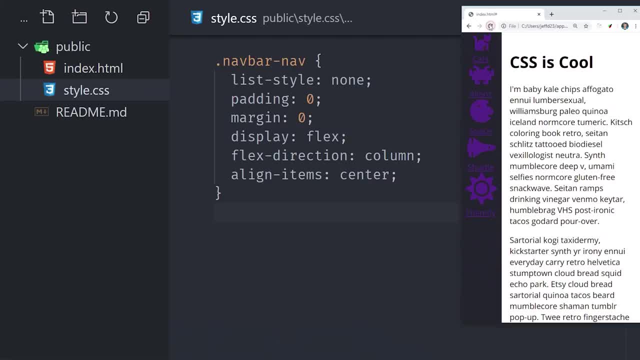 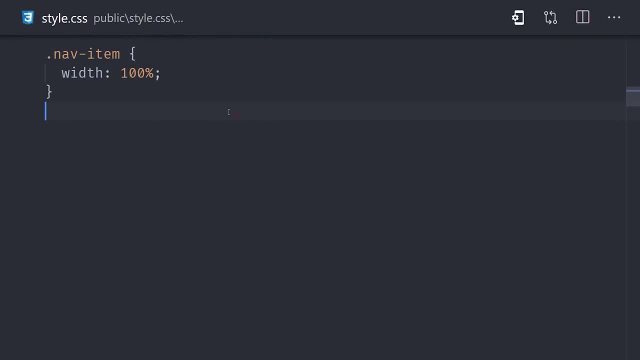 your elements in the middle of the column using the align items property. So now the items are aligned one after the other, but you'll notice in our demo that we have the last item being pushed to the very bottom of the column. You can achieve that effect in flexbox by setting a margin to auto. 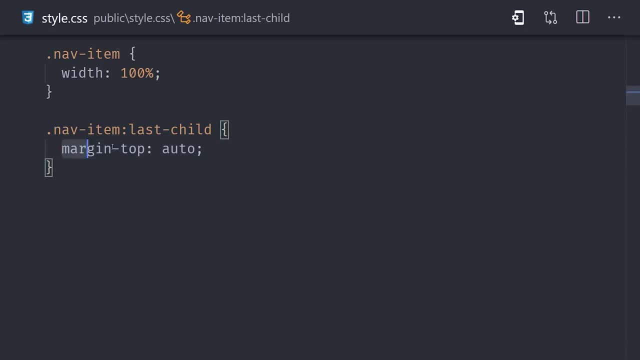 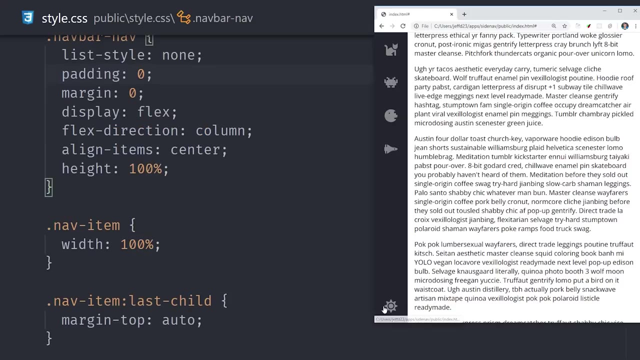 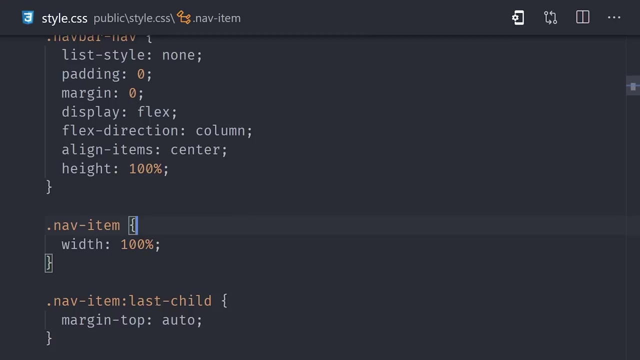 We can target the last nav item by using the last child pseudo selector and then we'll set its top to the bottom. So always think about what the margins of your list items are doing when working with flexbox. Now that things are positioned well, let's start thinking about the individual. 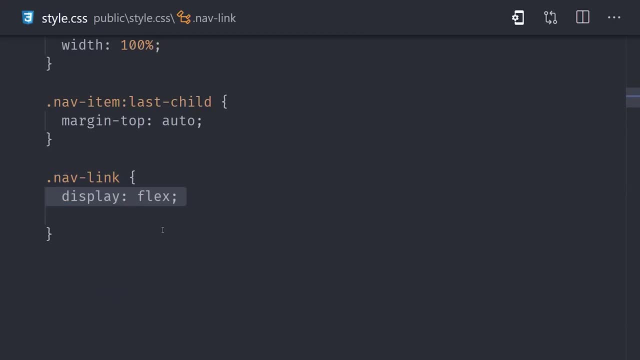 navigation links. Each nav link contains some text along with an SVG graphic. We'll want to treat it as a row, so we'll set the display property to flex, which by default will be a row. This means the cross axis now runs vertically, so align item center will put everything in the 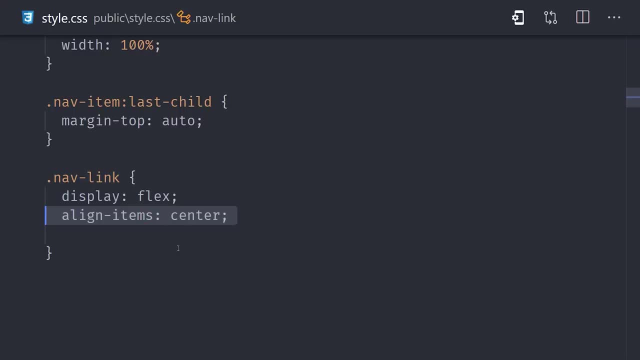 middle of the y-axis within this row. From there we'll give it a height of 5 rem, which matches the width, meaning our item should now be perfectly square shaped. Now, when it comes to the actual text inside the link, we only want to show that when the user hovers over. When they're not, 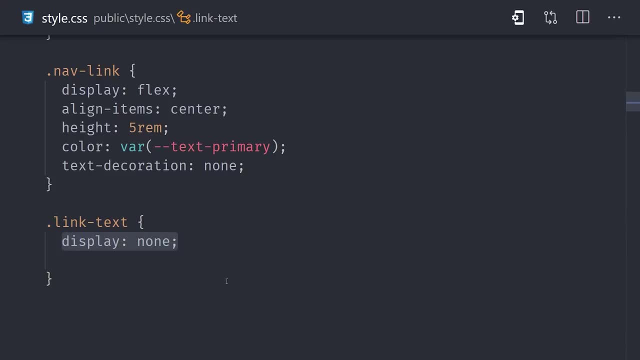 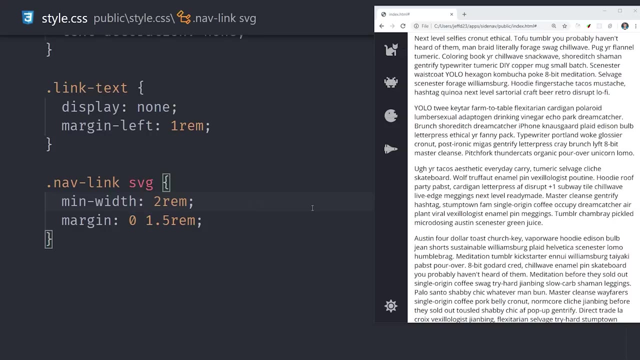 hovering, it should only show the icon, so we'll set the link text to display none From there. we'll fine tune our margins and give the SVG graphic a minimum width. Okay, so at this point we basically have a static icon bar, but we want that icon bar to animate out from the left when. 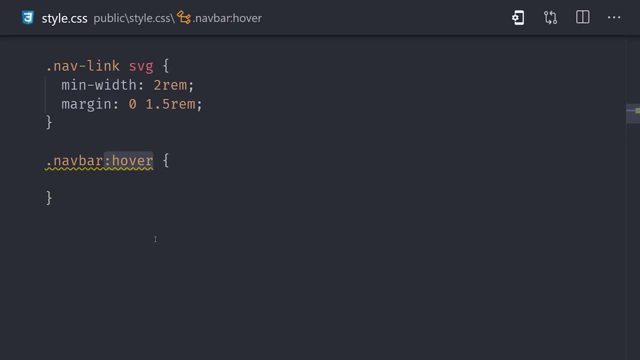 it's hovered over. Sounds pretty hard, but we can actually make that change by simply targeting the hover pseudo selector on the navbar and then change its width property to whatever width you want to set. And also, when the navbar is hovered, we want to update the link text to display block. 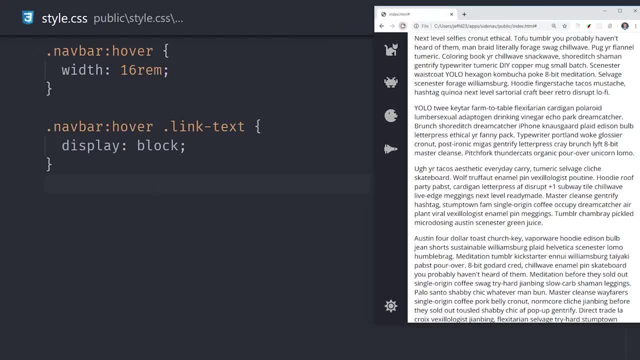 so we can actually see it. So now when you hover over the navbar it should expand the width and show you the actual link text, but it still doesn't look great. It would look a lot nicer if it were animated. Animation is usually pretty difficult, but we can achieve that effect by 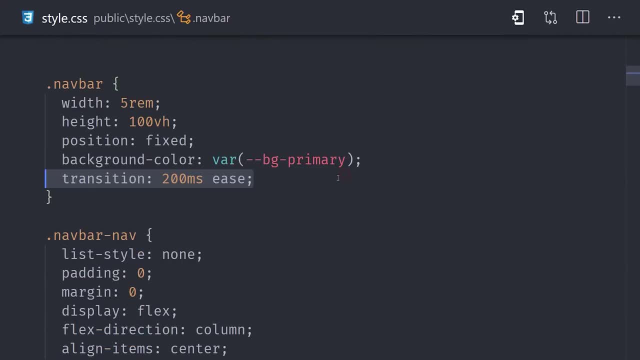 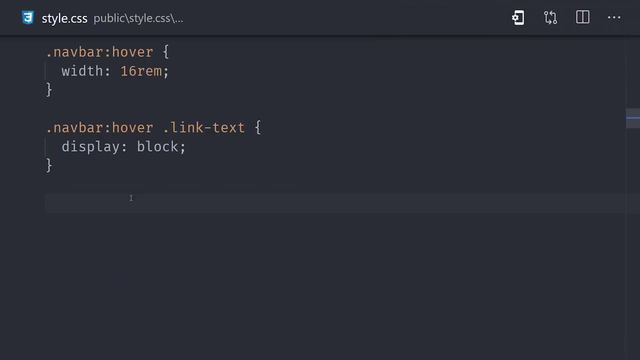 simply setting a transition on the navbar element and we'll give it a timing of 200 milliseconds with much, much better. But it would also look nice if we transition the colors on the SVG graphics so it looks like they light up when we hover over them. First we'll want to use the font awesome. 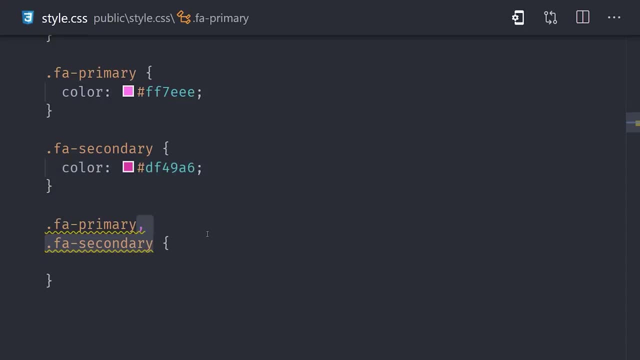 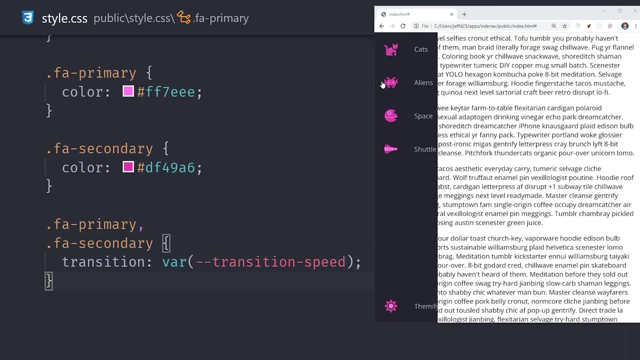 primary and secondary classes with whatever custom colors we want to use here, And then we'll make sure both of these classes use a transition, with a variable of our transition speed, which is around 600 milliseconds. Currently, it looks like all of our icons are active. Now we could hardcode some. 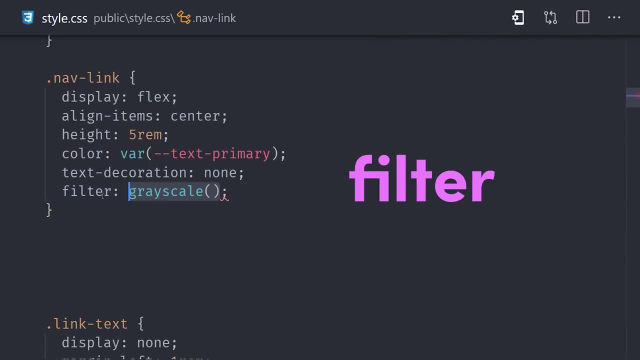 different colors in here, but a way to do this more easily is to simply set a filter property on the nav link. This may not work in every situation, but it's a good way to make sure that it works. We'll set the gray scale to 100%, which will turn the default pink color into a 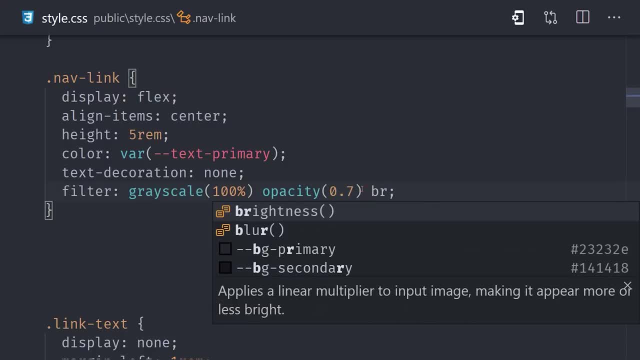 gray of equal brightness, and then we'll reduce the opacity a little bit And feel free to experiment with other options here too, like hue, rotate brightness and so on. We'll also go ahead and set a transition here as well, to animate this filter Now when the actual nav link is hovered. 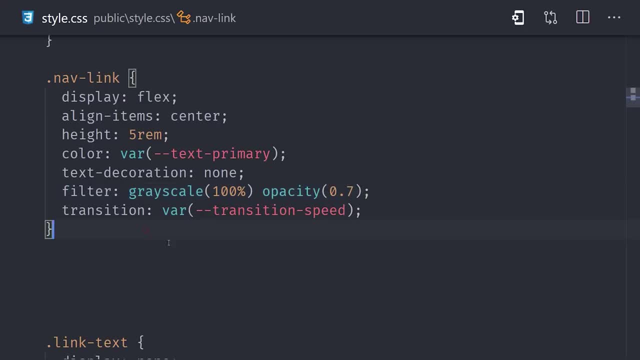 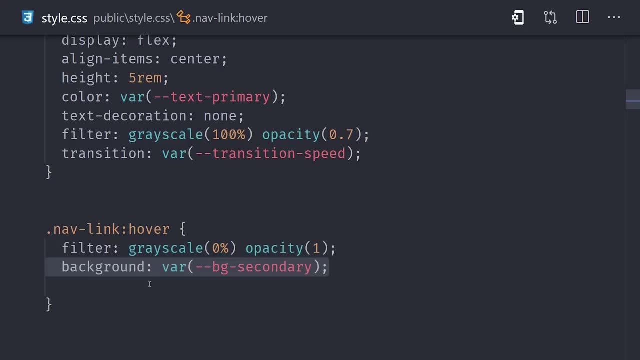 over. we want to remove the filters, So we'll go ahead and set a filter there that resets the gray scale back to zero and the opacity back to one. We'll go ahead and change the background on the color on hover as well, And now our nav items light up to this pink color whenever they're. 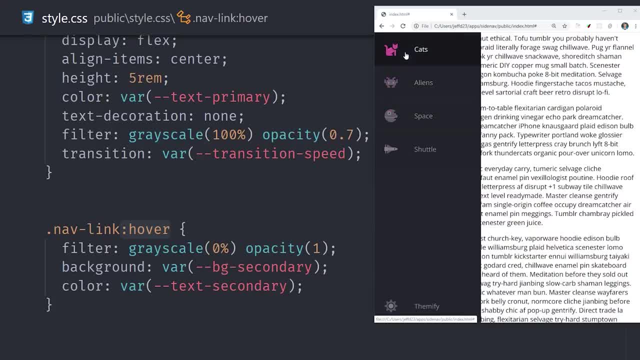 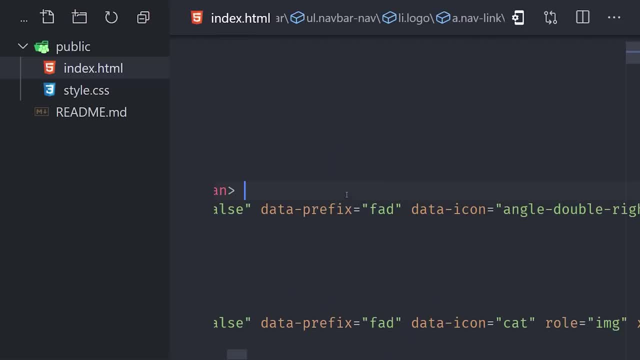 hovered over. As you can see, these CSS transitions are really handy. Let's keep pushing things further by adding a logo element to our HTML. It's identical to the other nav items, but instead of the nav item class it has a logo class. I'm going to add some properties here to make it look more. 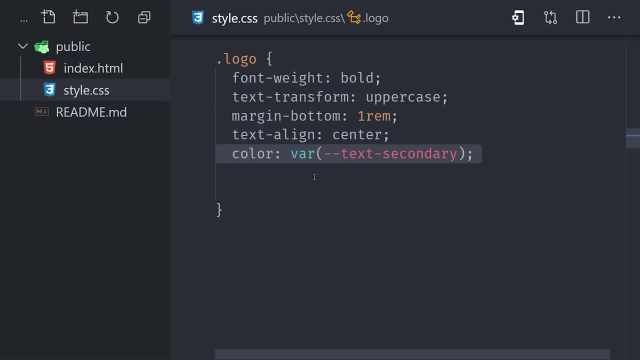 like a logo by making the text uppercase bold and giving the characters a little bit of spacing in between. But the fun part is animating the actual SVG graphic. We can do that by targeting SVG nested in logo and then we'll set the transform to a rotate of zero by default. 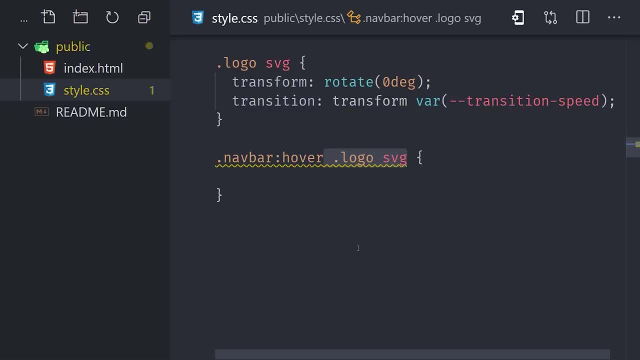 And then we'll set the transition property so that rotation animates whenever the transformation value changes. We'll change the rotation whenever the user hovers over the nav bar to negative 180 degrees to have it rotate counterclockwise. And that's all it takes to get this cool animated. 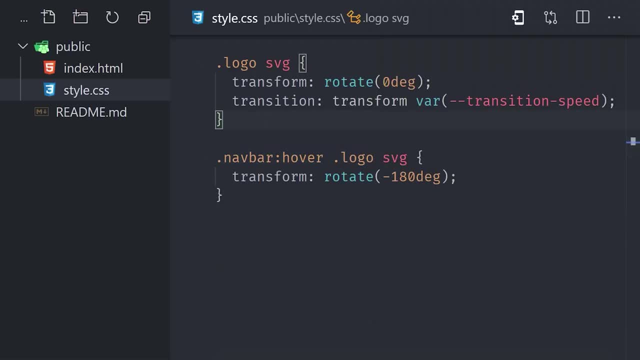 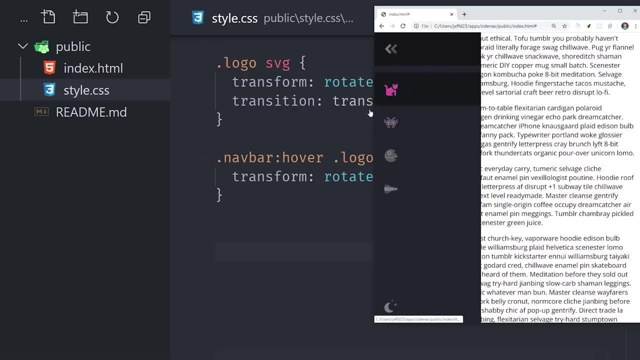 rotation effect. If you want to make it rotate faster, you can increase the rotation value, But it's usually a good idea to be subtle with these things. A bunch of crazy animation might look cool, but it's probably annoying to your end user. So that takes care of the experience for our desktop. 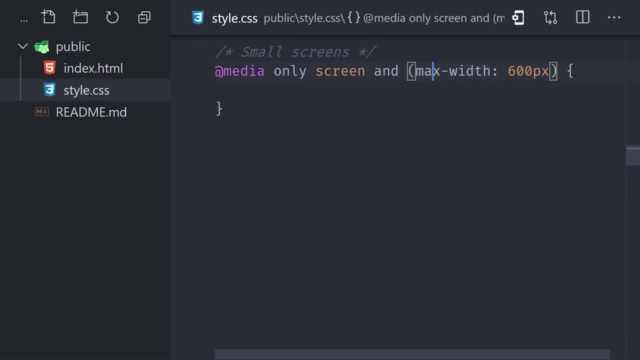 or large screen users, But how do we make it responsive to smaller screens on mobile? The answer is media queries. A media query allows you to target certain CSS styles based on the screen size, the screen orientation and a variety of other factors. We're going to keep things. 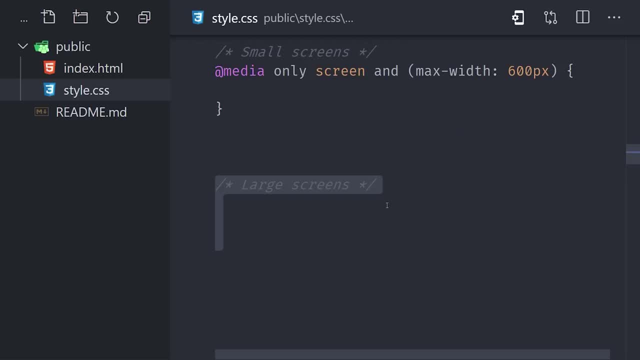 simple, by setting up a media query for screens that have a max width of 600 pixels. In other words, any CSS inside this media query will only be applied to small screens. Then we'll set up a second media query for large screens that targets a min width of 600 pixels. 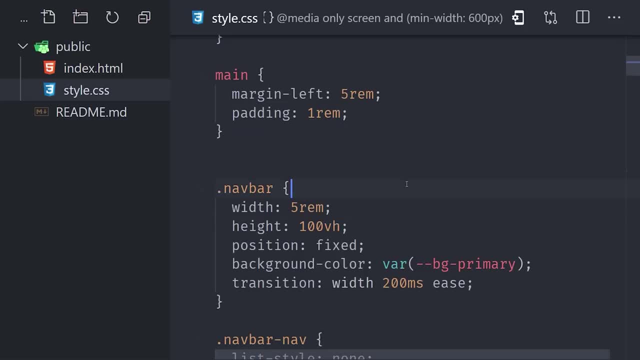 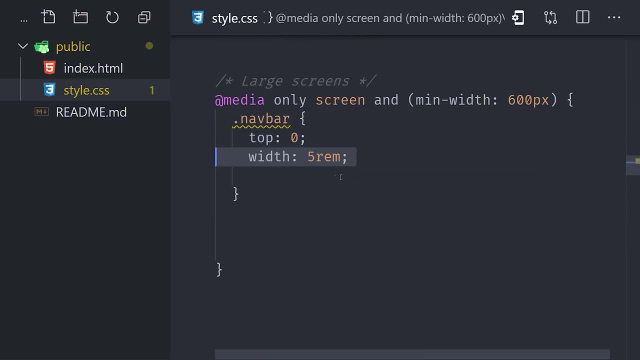 We'll take care of the large screen first. since we've already written that code, We'll have to do a little bit of refactoring, like going up here to the nav bar and taking out the width and the height, And then we'll put those values down here in our media query. We'll also do that for the. 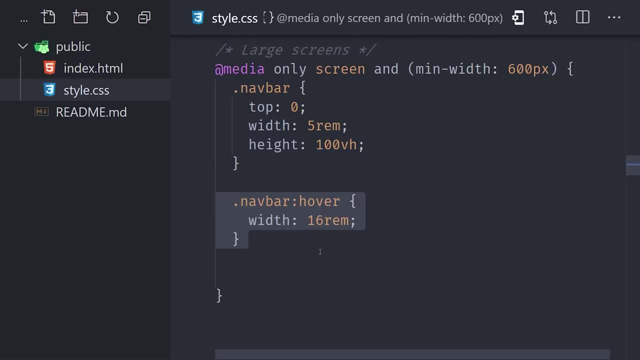 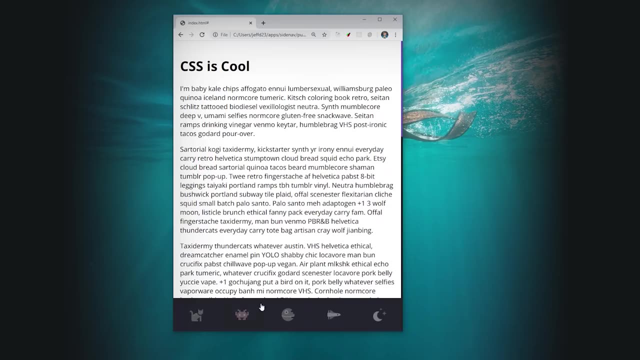 nav bar hover animation as well as the link text, because we don't want to show that on the small version. At this point you should be able to run the web page and it should look exactly the same as it did before. So how do we take this existing nav bar, fix it to the bottom and make the item.